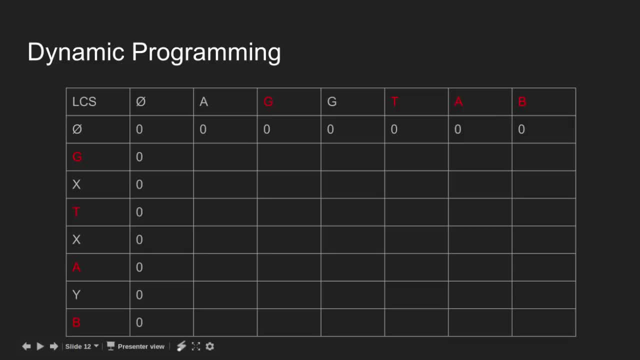 So we initialize the first row and first column with zero value. So we initialize the first row and first column with zero value. Now we move to the next row and compare G with the characters in the string AGGTAB. Since A does not match with G, we pick the maximum of the values stored. 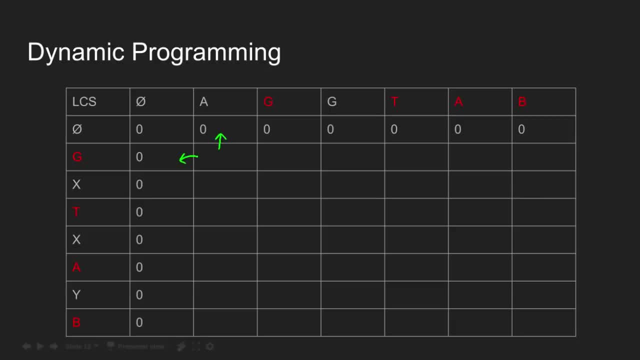 in the left cell and the top cell. Since G matches with G, we pick the diagonal cell value and increment it by 1.. So length of LCS becomes 0 plus 1, that is 1.. Again, G matches G, So length of LCS becomes LCS of diagonal cell plus 1, that is 0 plus. 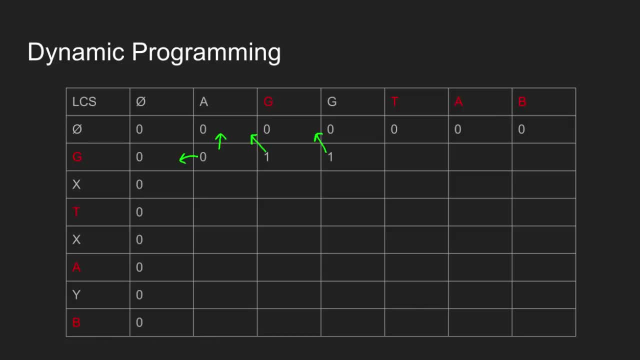 1 is 1.. G does not match T, So maximum of left and top cell is 1.. Length of LCS becomes 1.. Similarly, here 1 is the length of LCS, And here also length of LCS is 1.. So length: 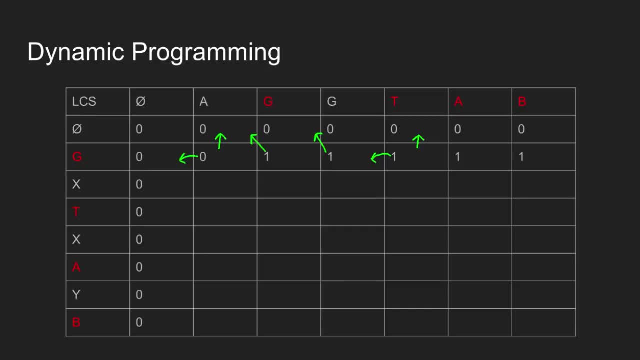 we will fill 1 for same reason. Now we move to the next row. X does not match A, So maximum of left and top cell is 0.. Length of LCS becomes 0.. Here X does not match G, So length of LCS becomes maximum of top and. 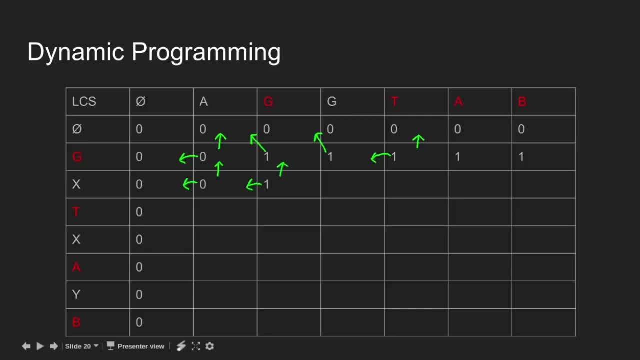 left cell, that is 1.. Since X does not match G, we pick the maximum of left and top cell, and L is 0. So length of LCS becomes 0. And here X does not match Tar, So length of LCS any character of the string a, g, g, t, a, b, we fill one in the remaining cells. 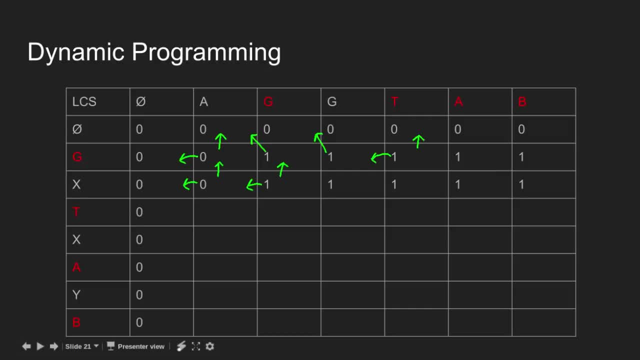 Now we move to the next row. t does not match a, So length of LCS is maximum of top and left cell. that is zero. t does not match g, So length of LCS is maximum of top and left cell. that is one. t does not match g, So length of LCS is maximum of top and left cell that. 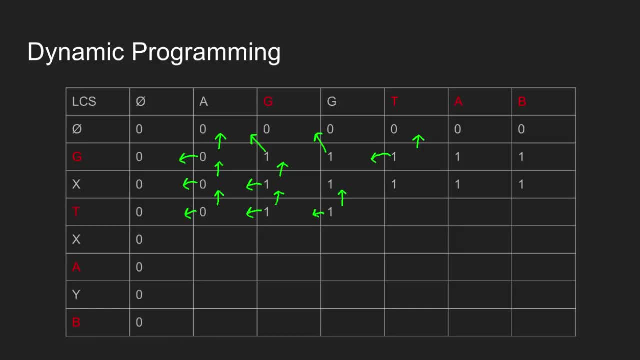 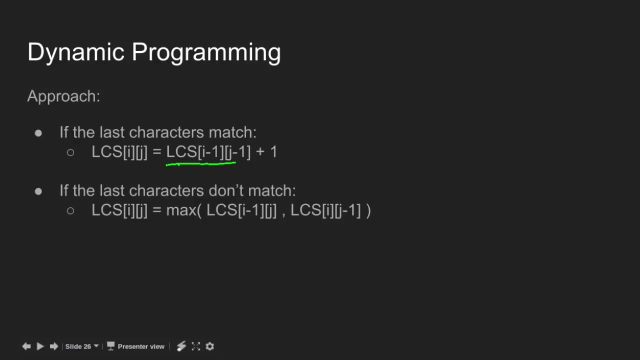 is one. Here t matches t, So length of LCS becomes LCS value at diagonal cell plus one. that is one plus one is two. We can fill the rest of the table following the same logic. In case of match, LCS of i and j is equal to LCS of i minus one, j minus one, which is the diagonal cell plus one. 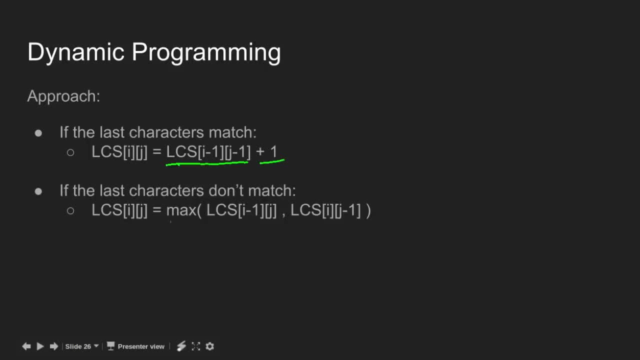 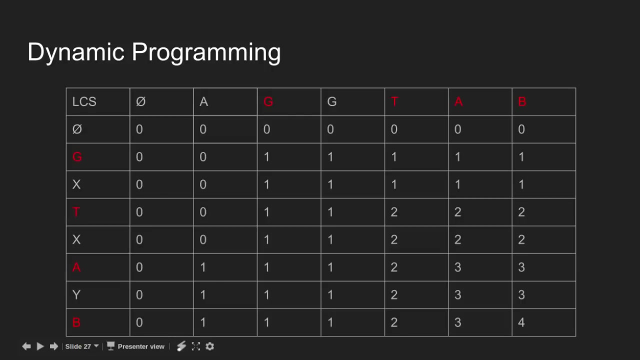 In case of mismatch, LCS of i- j is equal to maximum of LCS of i minus one, j, which is left cell, and LCS of i- j minus one, which is top cell. This is the final LCS table. Here, LCS of m? n is equal to four. 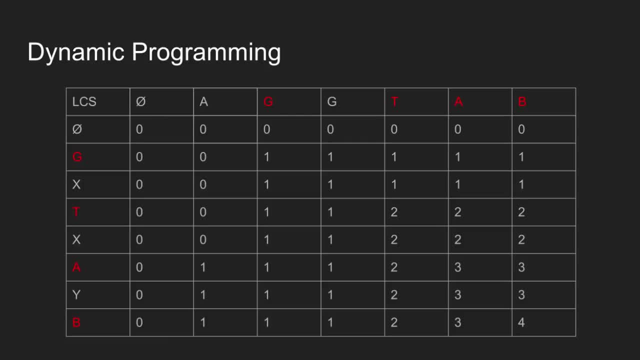 Here the interline of two получed twos and 4 is equal to four, Which gives us the length of the LCS of j. Let us see how we can obtain this LCS using this table. We start from the bottom right corner If we see that the stored value is not the 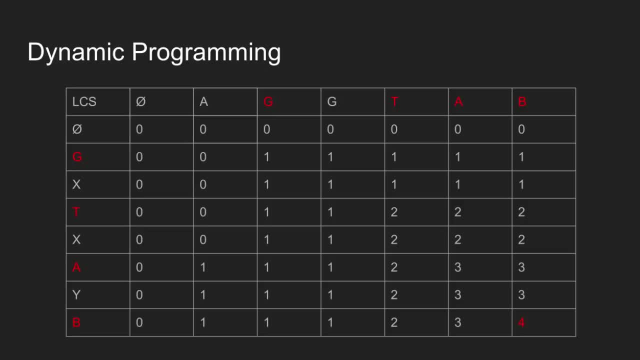 maximum of the top and left cell. it means the current character is a part of the largest common subseq. So we pick the character below on the left upper left-side of LCS of j b and move diagonally up. Since 3 came from top cell, we move up Since 3 is not the maximum. 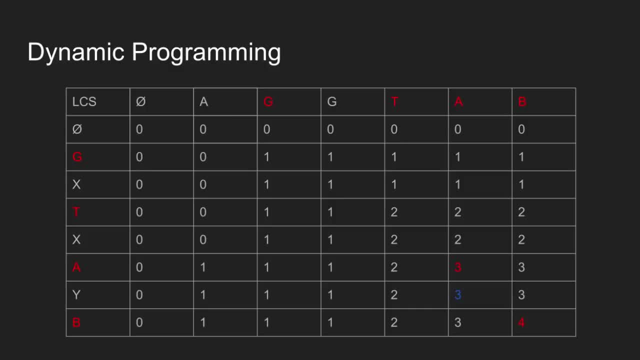 of top and left cell, we pick the character a and move diagonally up. Since 2 came from top cell, we move up again. Since 2 is not the maximum of top and left cell, we pick t and move diagonally up. Here 1 is the maximum of top cell and left cell, But this time both. 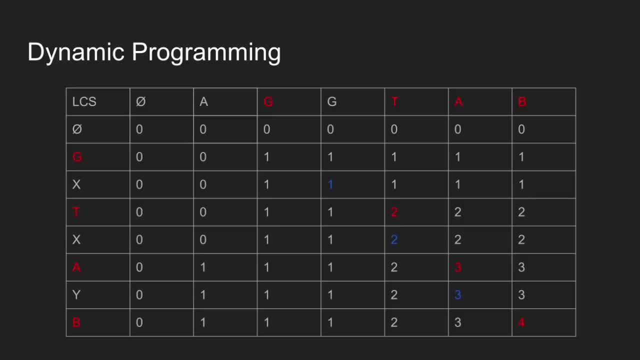 the top cell and left cell have the same value, So we can move in either direction. Let's move up. Since 1 came from left cell, we move left. Since 1 is not the maximum of left and top cell, we pick character g and move diagonally up. Since the stored value is 0, we stop.